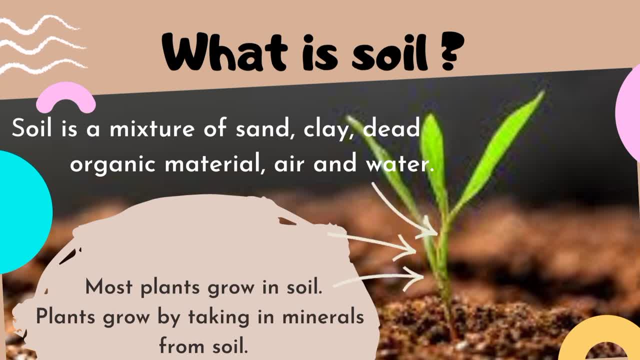 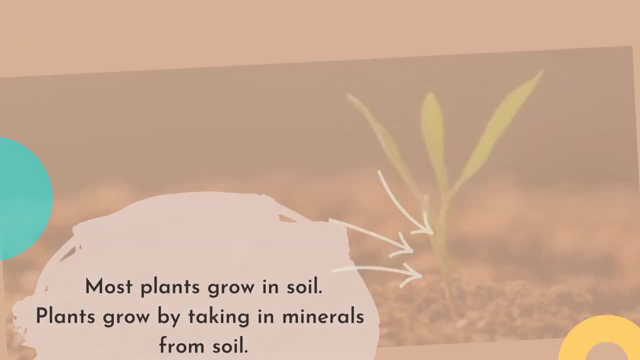 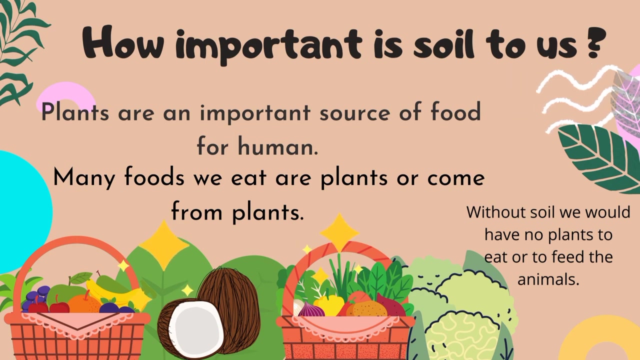 Did you know? most plants grow in soil. Plants grow by taking in minerals from soil, such as tree and many more. Alright, How important is soil to us? Plants are an important source of food for human. We know many foods we eat are plants or come from plants, such as vegetable and fruit. 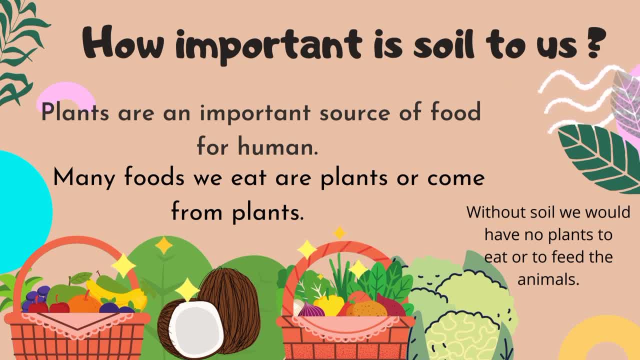 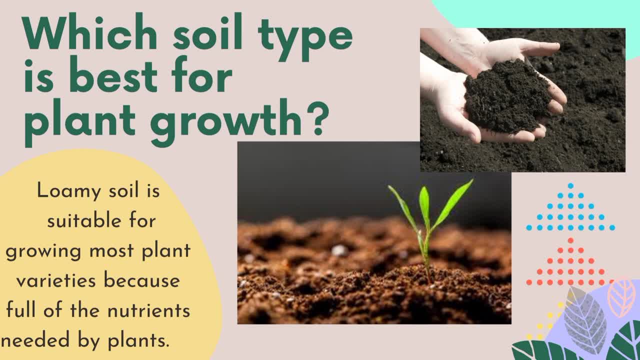 What can be found in soil? We can find dead plant or animal materials, water, sand, pebbles and also small animals like earthworms, termite and beetle. Which soil type is best for plant growth? The answer is loamy soil. 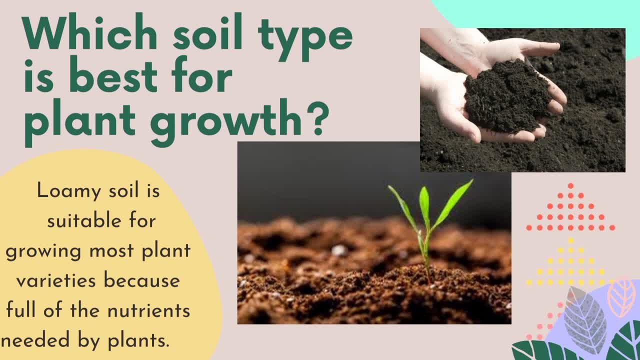 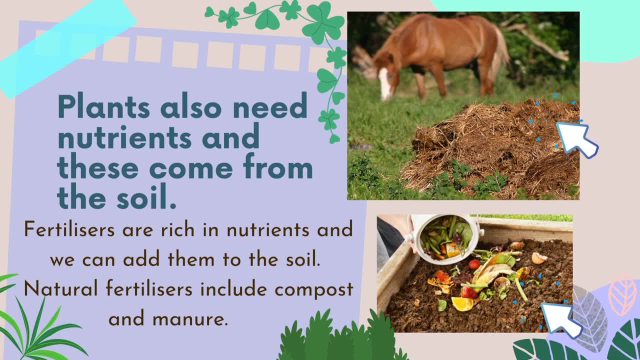 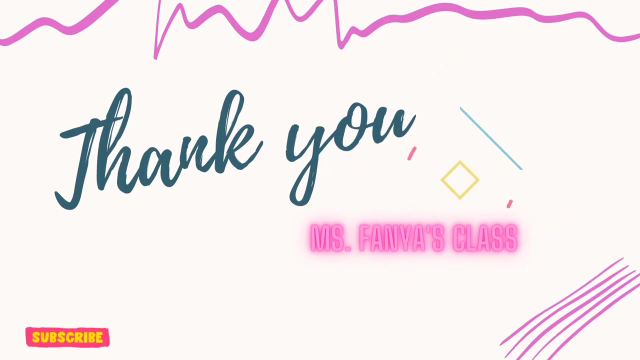 Why? Because loamy soil, full of nutrients needed by plants. full of nutrients needed by plants. not only humans. plants also need nutrients to grow and nutrients this come from the soil. fertilizer are rich in nutrients and we can add them to the soil. natural fertilizer include compost and manure. 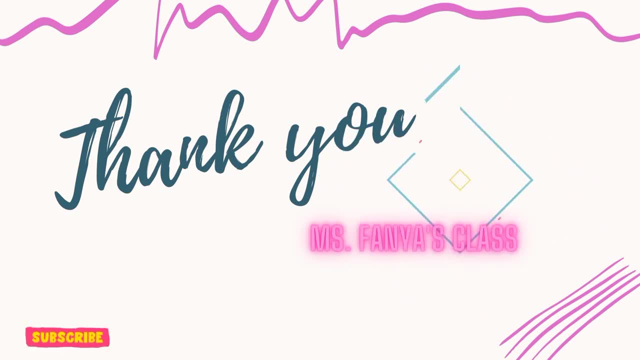 okay, everyone, I think that's all for today. I hope all of you understand about our topic today. thank you so much for your attention. see you on next video. bye.